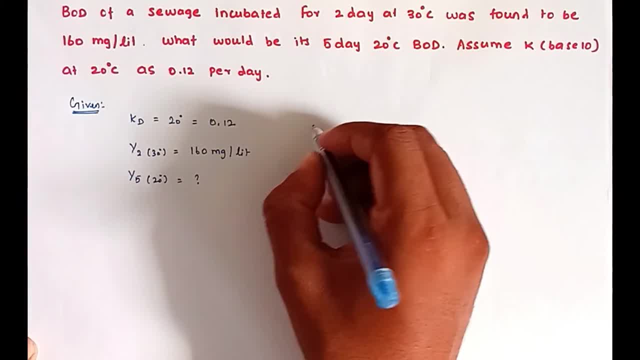 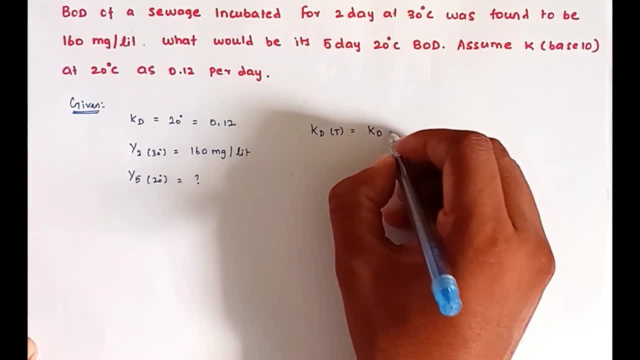 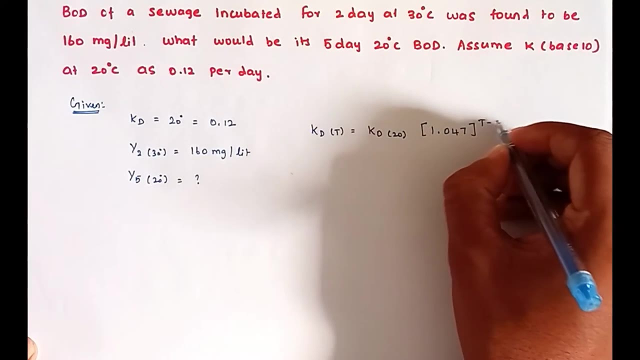 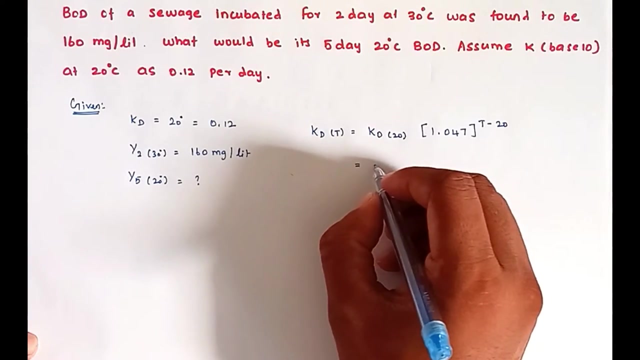 Okay, So we are going to find out the solution. So KD at temperature, the formula KD temperature equal to KD 20 degree Celsius, 1.047 power T minus 20.. So this is the formula. So now we can substitute KD 20 equal to 0.12, 1.047 power T minus 20.. 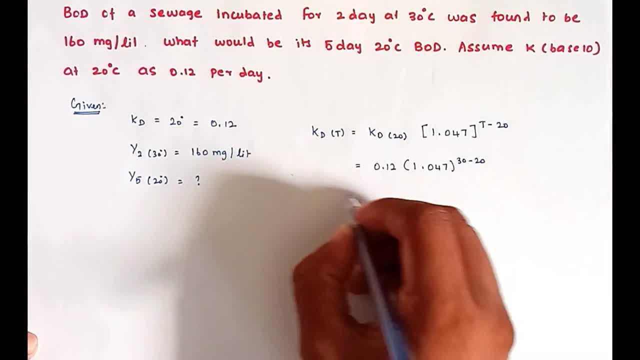 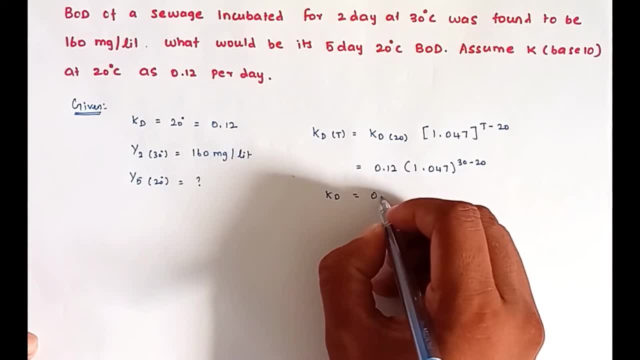 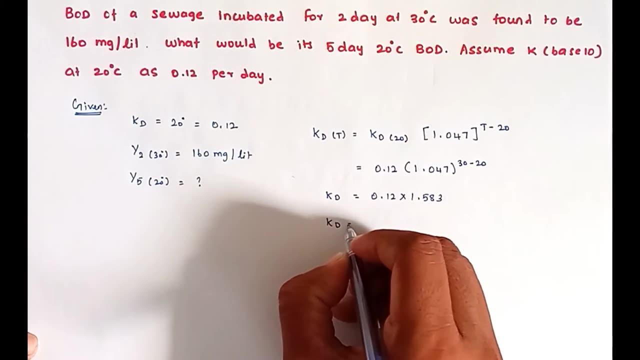 30 minus 20.. So now KD equal to 0.12, into dissolving this 1.583.. So now KD equal to 0.19.. So this is the answer. So next we are going to find out the BOD. 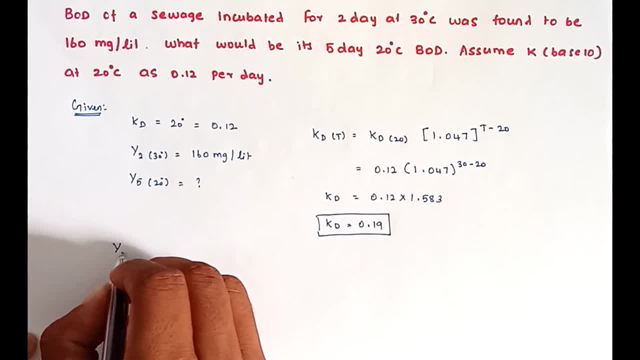 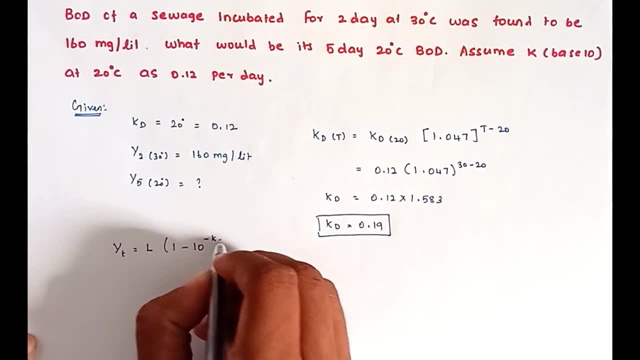 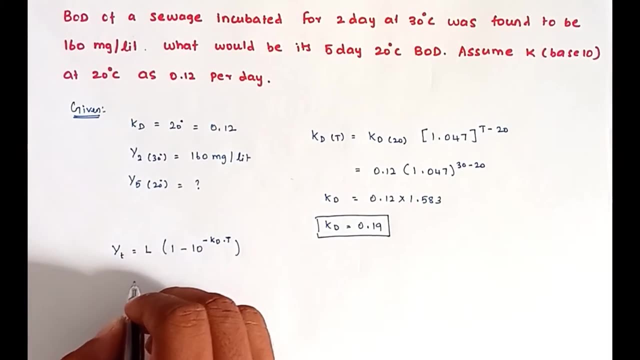 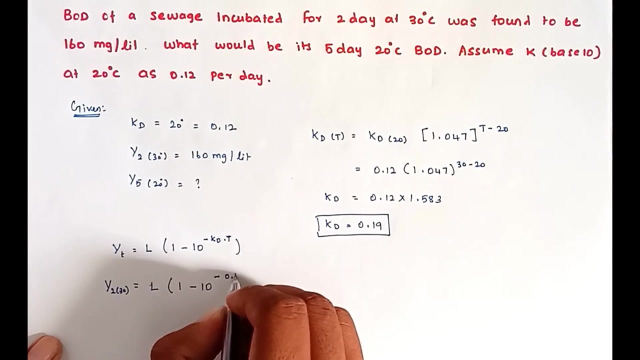 Okay, of 5 days, 20 degree Celsius. So the formula is: y, t equal to l into 1 minus 10, power minus k, t into t. So now we can substitute y to 30 into l, into 1 minus 10 minus 0.19 into 2.. So 2 days. So now, 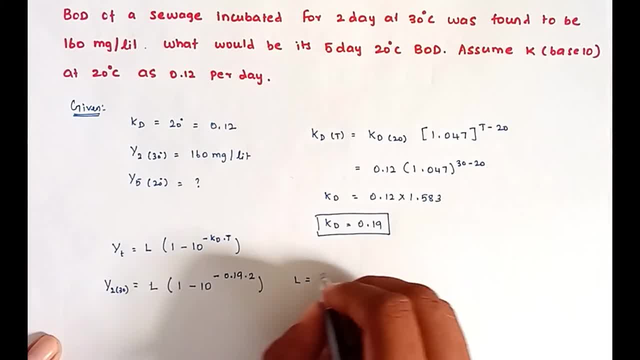 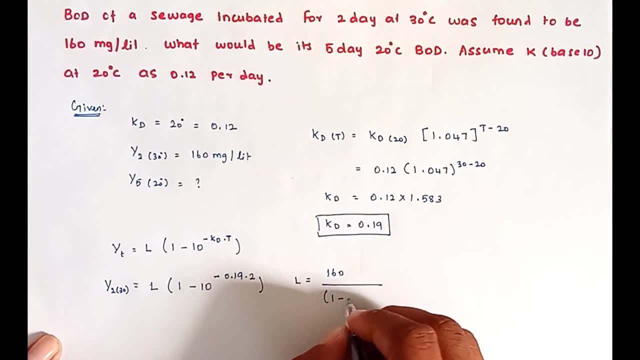 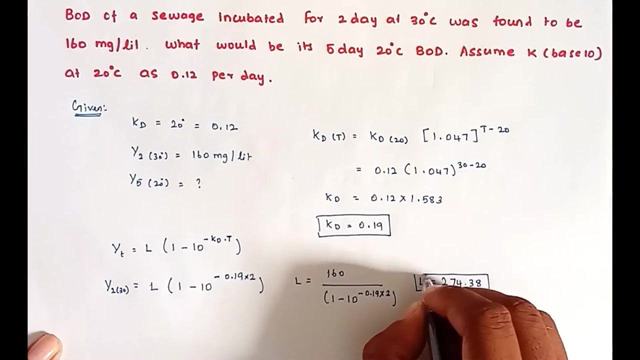 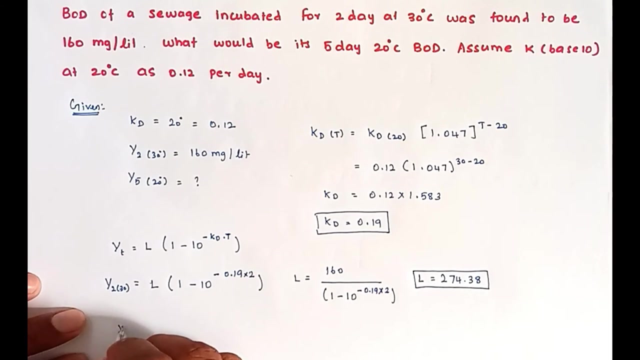 l equal to. so y to 30. is given 160 divided by 1 minus 10, power minus 0.19 into 2.. So now l equal to 274.38.. So again, we are going to substitute this l value to this formula, So y to 30. 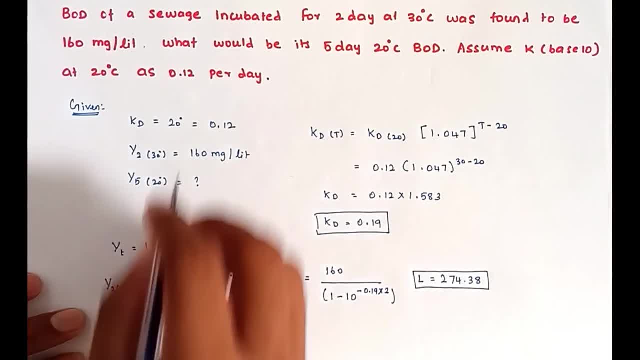 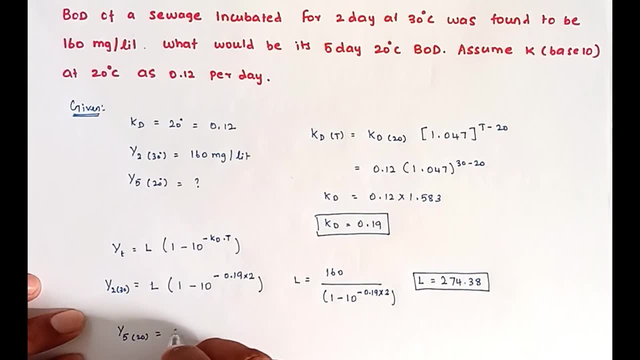 equals to y to 30.. So this l value is applied to y t, So it can be: this is v to 30 in order tov this z, little else. So v of z is equal to V t, D x equals to 5 times y t. So I am putting myself in this pop up like this, So something.